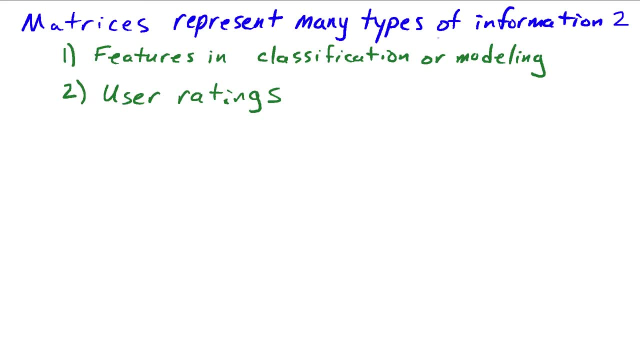 now that matrices can represent many types of information. We've looked at features in classification or modeling. We've looked at users' ratings of things like movies or products. We can also use matrices to represent collections of documents, For example. one approach is to use 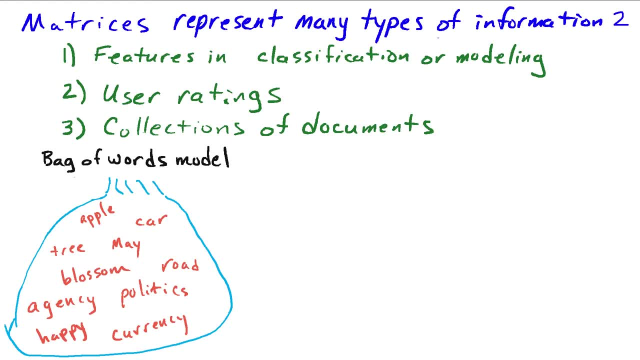 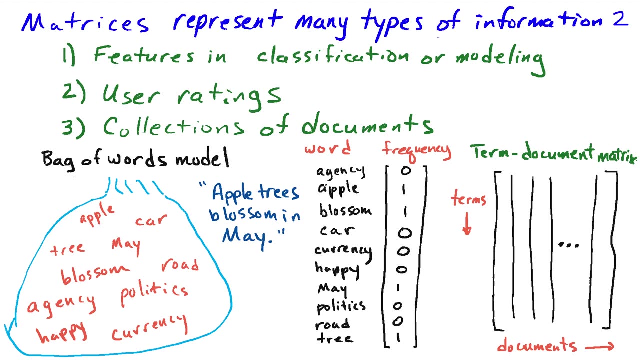 a so-called bag-of-words model, where you just count the number of occurrences of each word in a particular document and put those counts in a vector. So you're ignoring the relationships between words, You're simply counting the words that are in the document. For example, if I have 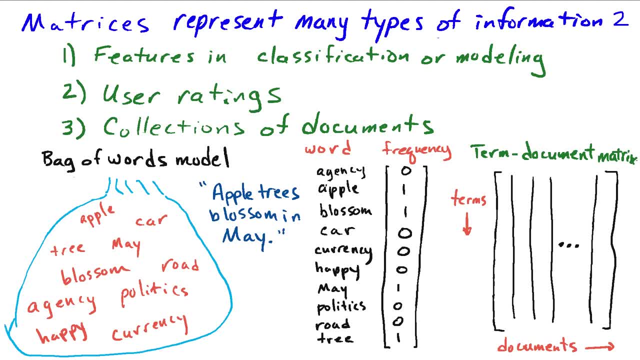 the sentence apple trees blossom in May. I can count the frequency of the words in that sentence. So agency does not occur in that sentence. It has zero frequency. Apple occurs once, Blossom occurs once, Car does not occur, Currency does not occur, May occurs And politics. 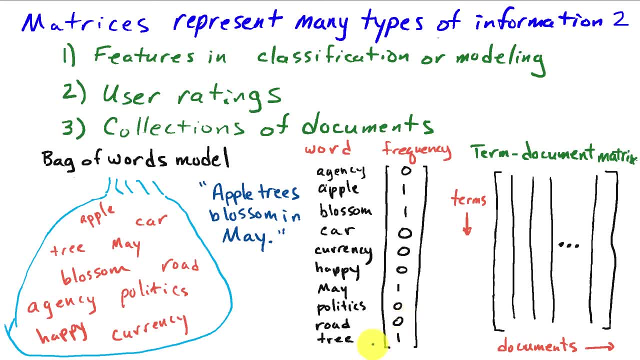 and road do not occur And tree does occur. If I have a dictionary of words that I'm considering, then I can count the frequency of each word in a document and represent that document with that vector. And if I stack a bunch of words in a vector I can count the frequency of each word in a. 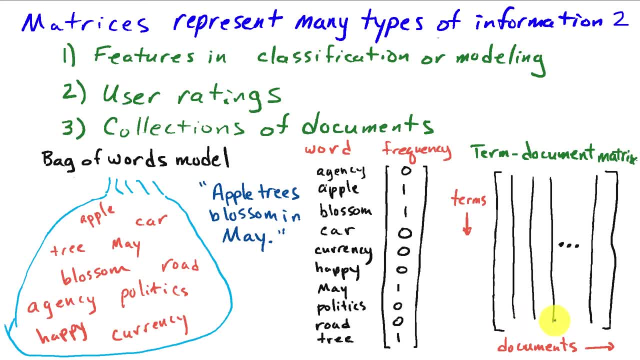 vector. If I have a dictionary of words that I'm considering, then I can count the frequency of each of those vectors as columns into a matrix. I have what's called a term-document matrix, So the terms go down the rows- That's the count of each term or word, And then across the columns. 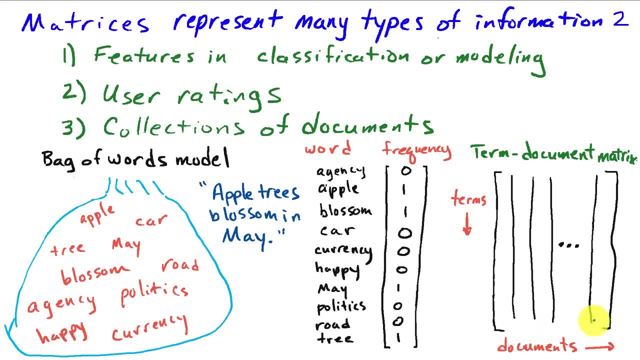 I have different documents And by studying the structure of this matrix we can infer things about the relationships between documents, similarities, We can perform queries to look for certain terms and so on. Now, low-rank decompositions of some of the terms that are in the document are the ones that are in the document. So 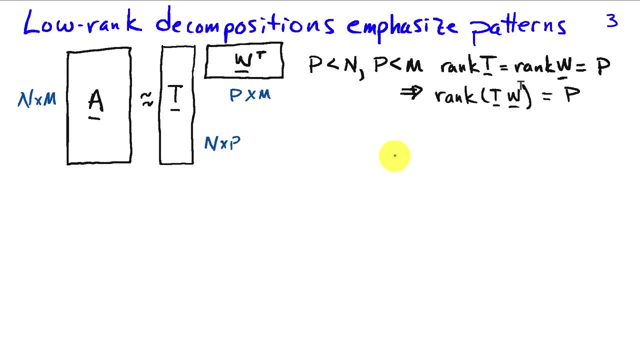 such matrices emphasize patterns, And that's the main purpose of these is to identify dominant patterns that we can use in our subsequent machine learning. So let's take an n by m, matrix A. So it says n rows and m columns. A low-rank decomposition represents that matrix as the 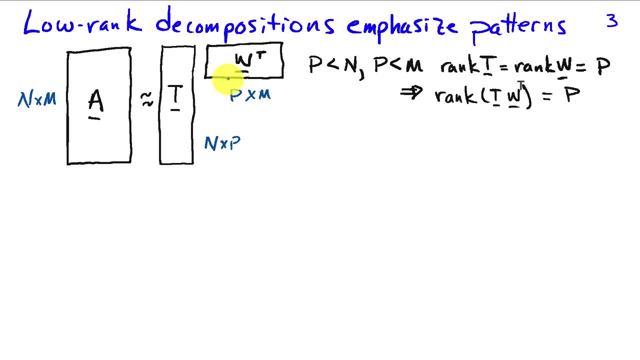 product of an n by p matrix T and a p by m matrix W. transpose In general: p is going to be less than n and p is going to be less than m. Oftentimes, p will be significantly less than both n and m. Now, if the rank of T and the rank of W are both p, then the rank of this 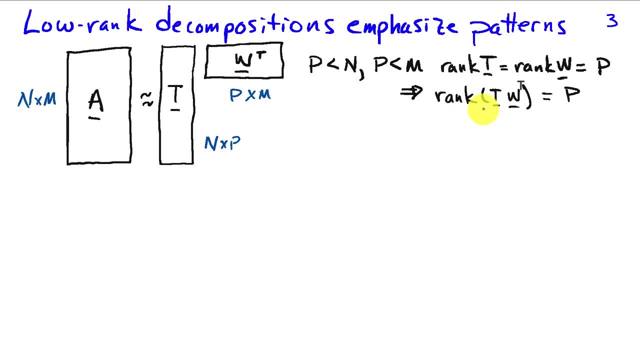 product T times W. transpose is also p And in general A could be rank as large as the minimum of n or m. So p being much smaller than those represents a low-rank approximation or a low-rank decomposition of the matrix A. So we're going to define the matrix T in terms. 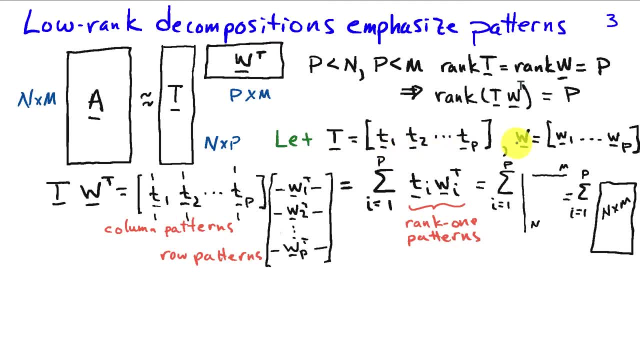 of its columns T1, T2, through TP and a matrix W in terms of its column W1 through WP And then T times W transpose can be written as the outer product of a series of column patterns associated with the Ts times, a series of row patterns associated with the rows of W transpose. 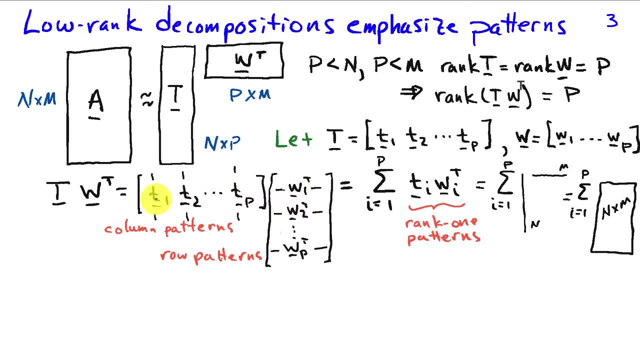 and so on. So when I do this multiplication, I have T1 times W1 transpose plus T2 times W2 transpose, and so on, And I see that I can write this as a sum of: I equals 1 to p, T, I, W, I. 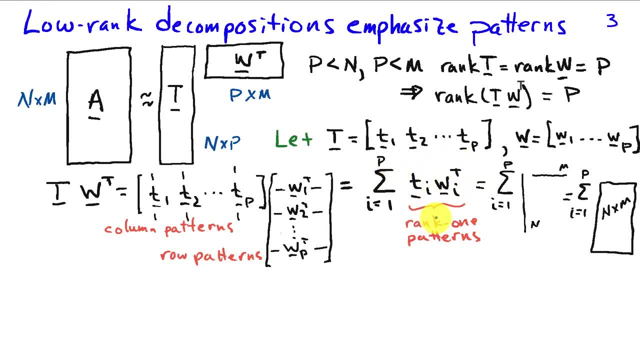 transpose and each of these products is a rank 1 matrix because it's a product of an n-dimensional column times an m-dimensional row vector And that results in an n by m matrix. In this form we're writing A as a sum of these rank 1 pattern matrices. A really important question. 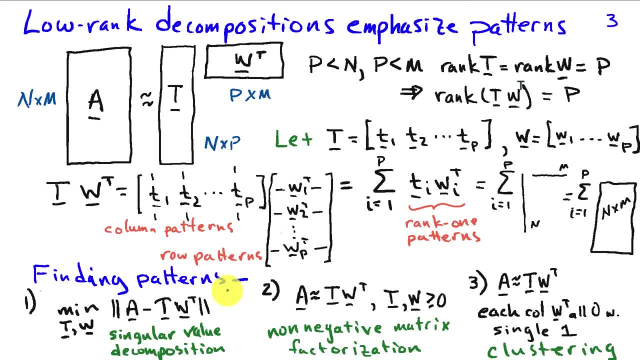 is: how do you find good patterns- T and W- to do this kind of low-rank decomposition? And there are multiple approaches to this problem, three of which I've listed here. So one approach is to say that you want to find the T and the W transpose that are rank p, so that this product T, W. 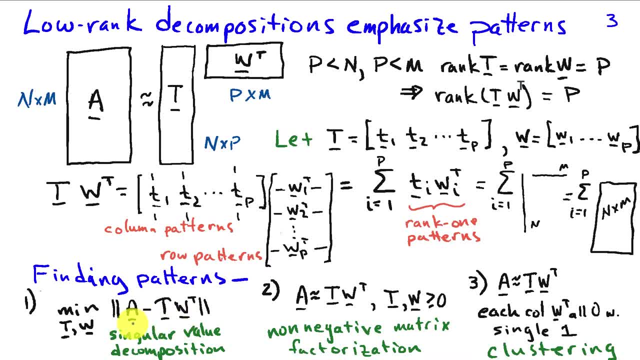 transpose is the closest possible to the matrix A in the sense of some norm, And we'll look at a specific norm and find that this leads us to the topic of singular value decomposition of the matrix A. Yet another approach is to factor A in terms of a product of matrices T and W transpose, where all the elements 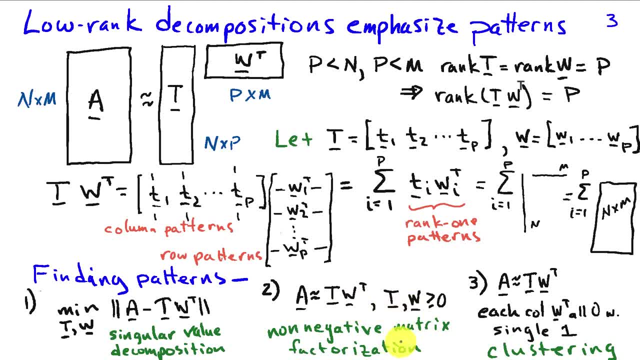 of these matrices are non-negative. This is a so-called non-negative matrix factorization and is very useful in certain problems where A contains positive entries, such as the term document matrix or a ratings matrix. Yet a third approach is to restrict the matrix W transpose so that each column contains all zeros but has 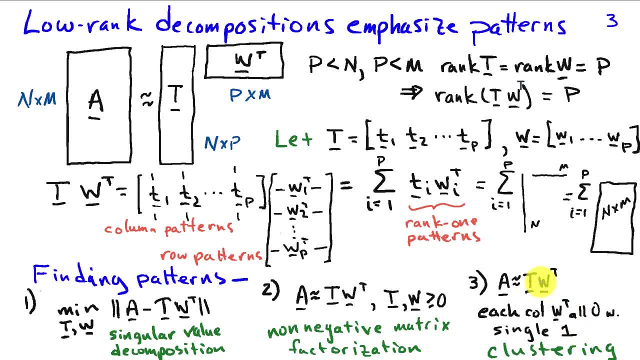 a single 1.. So let's suppose there's a 1 in the k-th row of W. transpose: Well, what that's going to do is pick out the k-th column of T. Therefore, we're approximating each column of A, in this case by a particular column of T, And this is a so-called clustering problem. 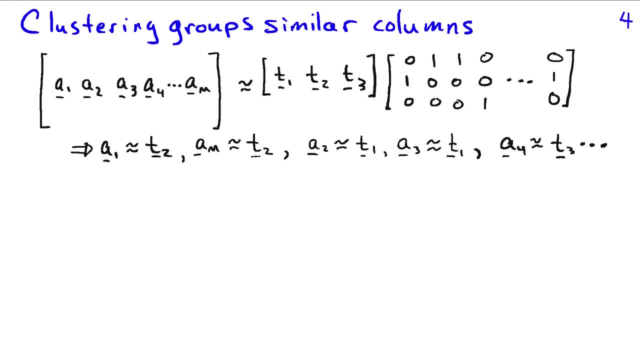 So let's explain this clustering idea in a little more detail. Suppose I have a matrix whose columns are A sub i, so A1, A2, A3, so on up to A sub M, and I'm going to approximate that matrix as a matrix T, which in this example we'll assume T has three columns In clustering. 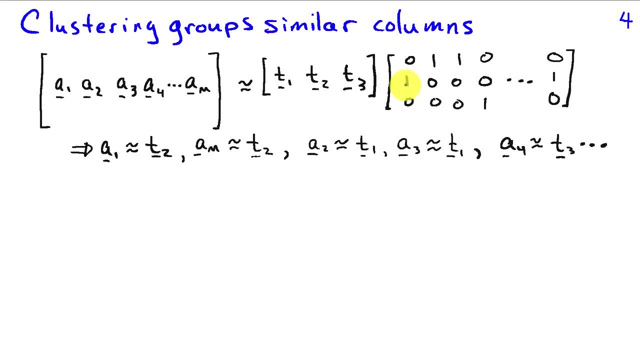 the matrix W transpose has a single one unit. Well, K is an initial matrix, but it's not in each column and the rest elements are zeros. So, for example, I might have 0,, 1,, 0, and if I 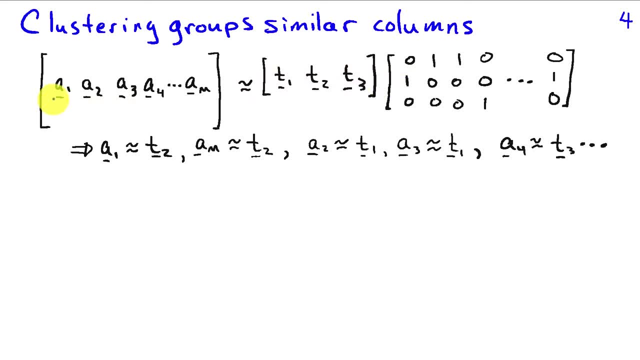 multiply these out, this tells me that the first column, A1, is equal to 0 times T1 plus T2 plus 0 times T3. So A1 is being approximated by T2.. Similarly, if I go down here to AM, AM 0 times. 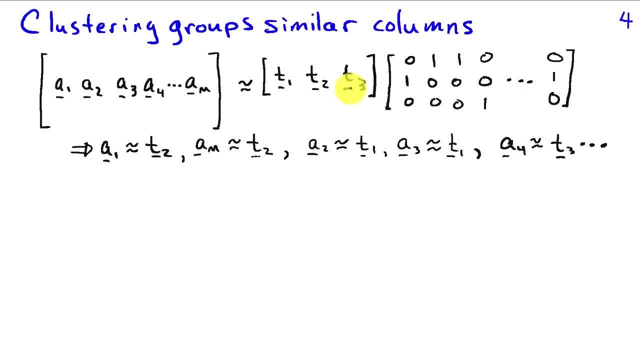 T1 plus 1 times T2 plus 0 times T3, in other words, A sub M is also being approximated by the column T2.. And similarly we can look at the other columns and the way I have this set up in this example. 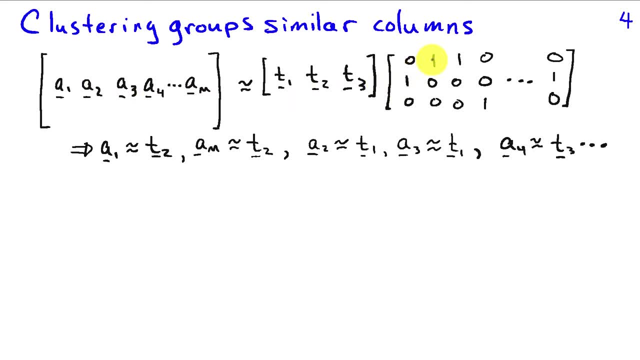 the second column, A2, is being approximated by T1,, as is the third column, because there's ones in both of these cases. And then the fourth column of the matrix, A- A4, is being approximated by T3. 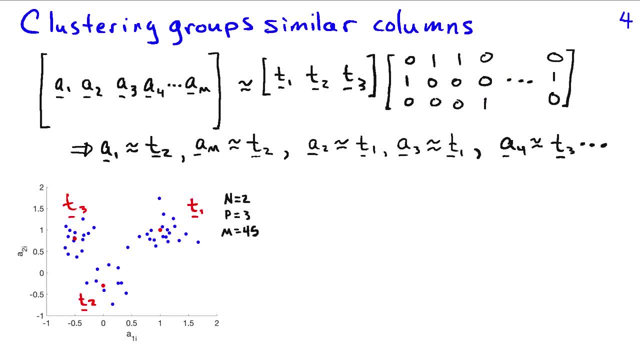 and so on. If I draw an example of this in two dimensions, so this would be: N equals 2, and we'll assume that there are P equals 3 clusters like I've drawn here with T1, T2, and T3.. In this case, I've chosen M. 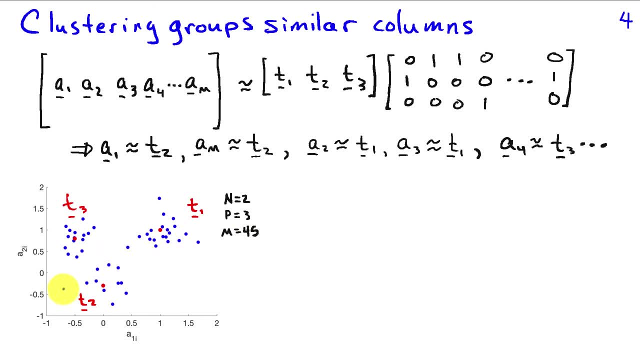 to be 45. You can see that this data maybe could be represented by three clusters: one here that's T2, another that's clustered around T1, and a third that's clustered around T3.. So what we'd like to do is we're going to do a little bit of a study of this. So we're going to do a little bit. 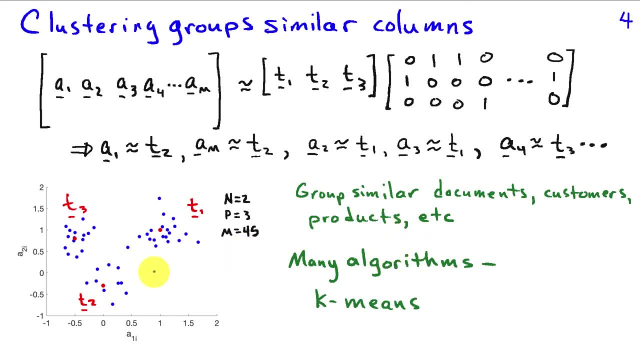 of a study of this. So what we'd like to do is take a matrix of measurements- all 45 data points that are represented in this two-dimensional problem, and then we'd like to group the ones that are similar, In other words, assign cluster centers to those and that could be representing. 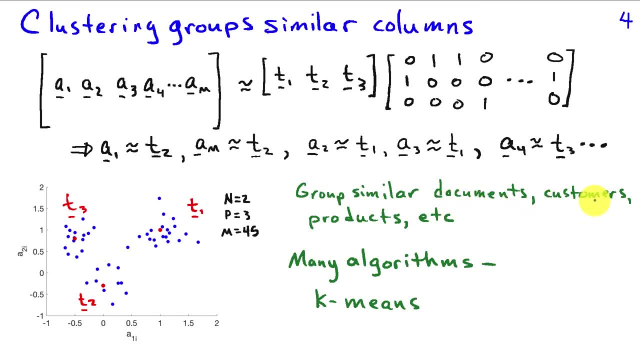 similar documents, grouping customers that have similar preferences, grouping products that have similar attributes, and so on. Now, there are a lot of different algorithms for doing this kind of clustering. The first one is the k-means algorithm, and that's something that we'll look at in detail in a 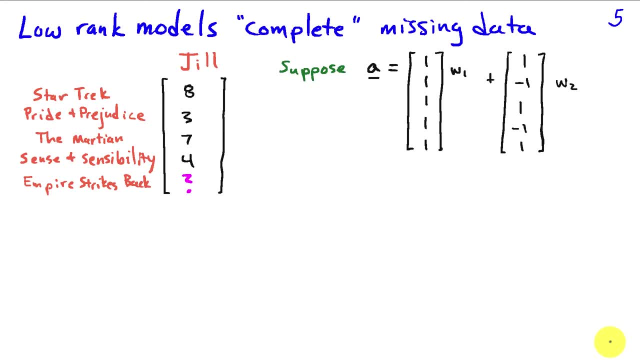 subsequent lecture. Now, something else you can do with these low-rank models is complete missing data. For example, suppose we have these five movies: Star Trek, Pride and Prejudice, The Martian Sense and Sensibility, The Empire Strikes Back, and Jill has watched four of those and we'd like. 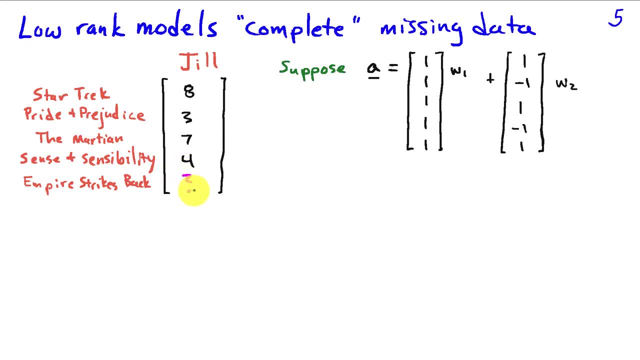 to make a prediction what her rating is going to be. for the fifth one, The Empire Strikes Back. We're going to assume a model that our ratings are given by the sum of two terms: an average term which has ones in all of the different elements, and then we're going to assume that people have different preferences. 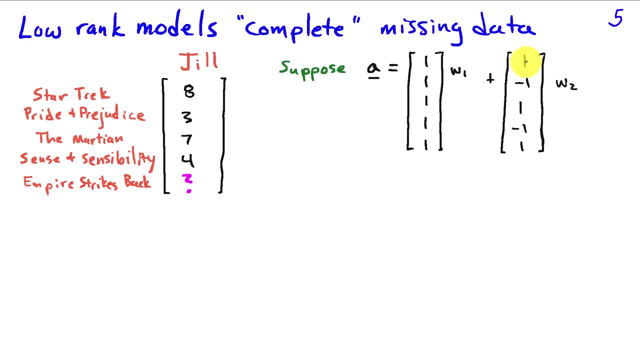 for science fiction movies versus romance movies. So we put ones here in our second column of t in the positions corresponding to the science fiction movies, and we put minus ones in the positions corresponding to the science fiction movies. So we're going to assume that people have 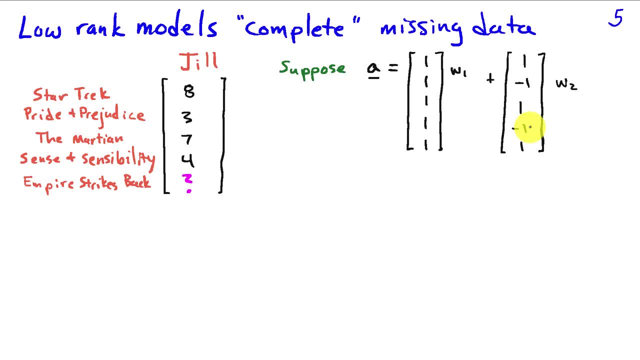 different preferences for the romance movies. So if someone preferred romance movies over science fiction movies, w2 would be negative and that would increase their ratings of the romance movies relative to the science fiction movies. So in this case we're assuming we know these two. 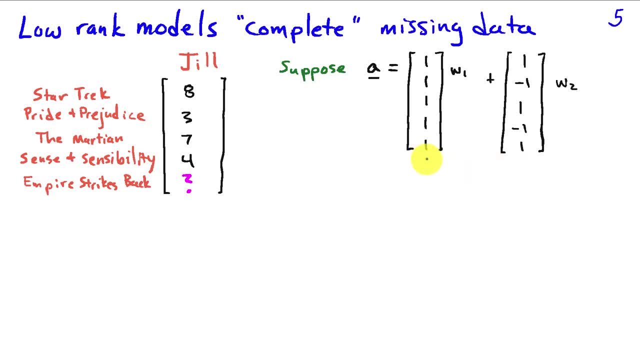 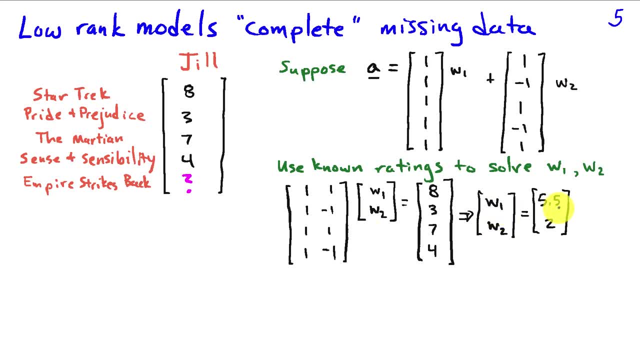 the least squares problem and you find that w1 is 5.5,, which happens to be the average of these four ratings, and w2 is 2.. Well, once we have w1 and w2,, we can then predict the ratings. 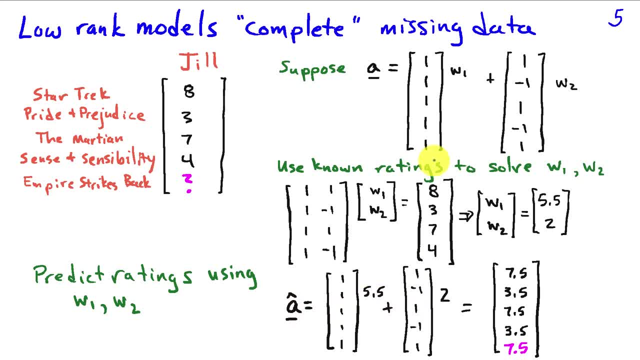 and we'll call that a hat. using w1 and w2 and these low-rank bases, t1 and t2, for this five-dimensional space representing ratings, We find that we predict Jill's ratings to be 7.5, 3.5, 7.5, 3.5, and 7.5. Thus, we would predict that Jill is probably going to like the. 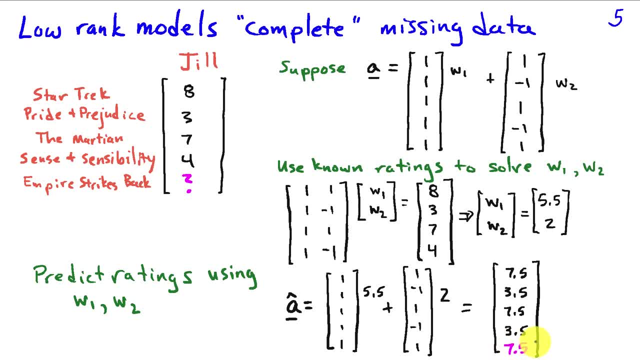 science fiction movie The Empire Strikes Back. Now, you'll note, in this case, each of these categories has just been replaced by the average rating for their category in this prediction, and that's because we used only two taste profiles or basis vectors to represent these ratings. 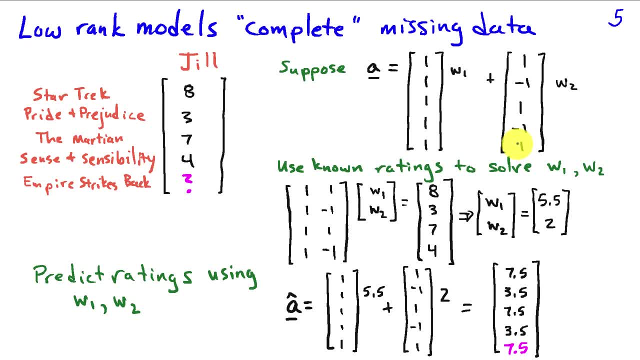 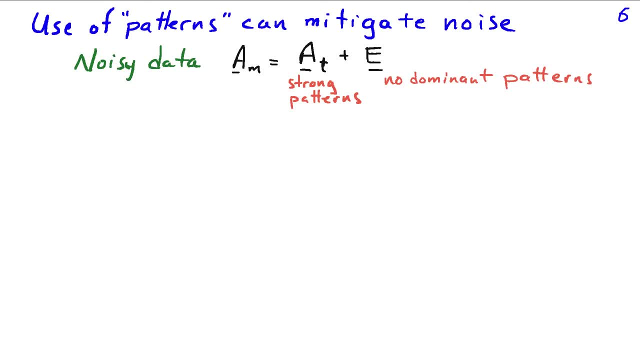 In general, if one had a more complex problem with a lot more data, you would end up with more diversity in your ratings. Now, another benefit of this low-rank approximation is that, by relying on the dominant patterns, we can mitigate the impact of noise, For example, let's suppose I'm collecting 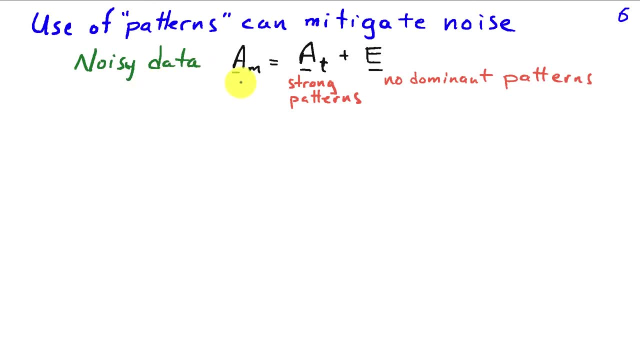 features for a classification problem or a modeling problem, and there's noise present. So I have underlying features that I can't measure, which have strong patterns in them, and then I have this noise, which really doesn't have any dominant pattern. So if that's my measured data, a sub m is noisy. 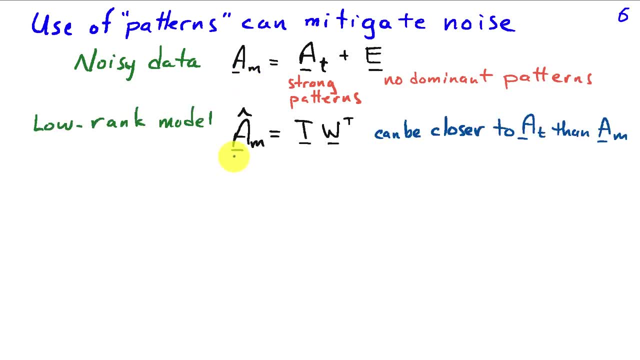 and I approximate this with a low-rank model, say t times w transpose, I can choose t and w transpose in such a way that this low-rank model ends up being closer to the true features in a t than to the measured data, a sub m, because our patterns can be very different. So if I have a, 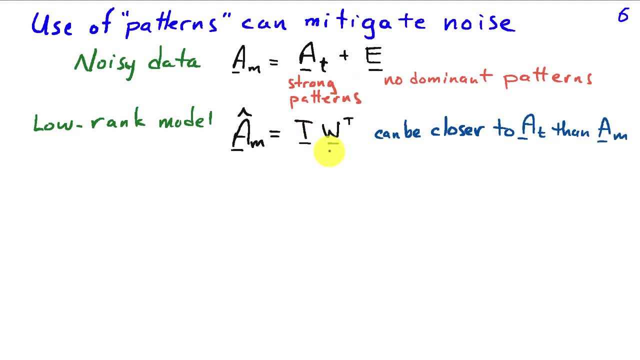 low-rank model. I can represent it by t, and w will clue in on the strong patterns in a t and not be influenced very much by the lack of structure that's present in the noise data. So then I can set up, say, a low-rank classification problem or a low-rank modeling problem by replacing a sub m. 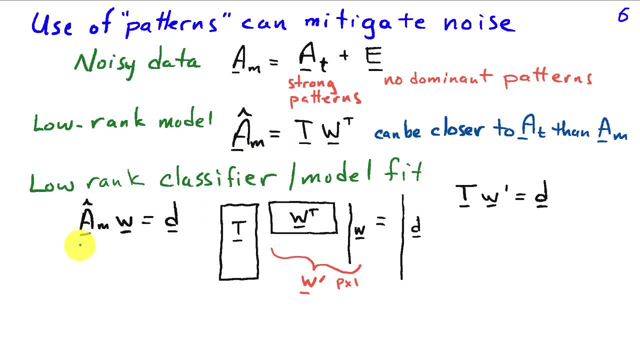 my measured noisy data. with my low-rank model We have the least squares problem. We're trying to solve a sub m hat. We have t times w is equal to d. Substitute a m hat in terms of its low-rank decomposition. We have 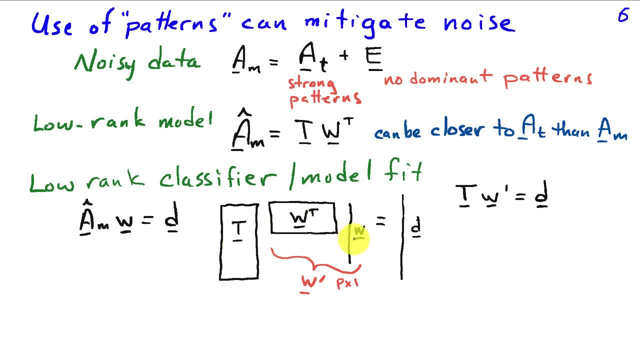 t times capital W transpose times lowercase w is equal to d, and we still want to solve this as a least squares problem. One thing that we observe is that, since w transpose is a known matrix, the product of capital W transpose and our m-dimensional vector, lowercase w, is: 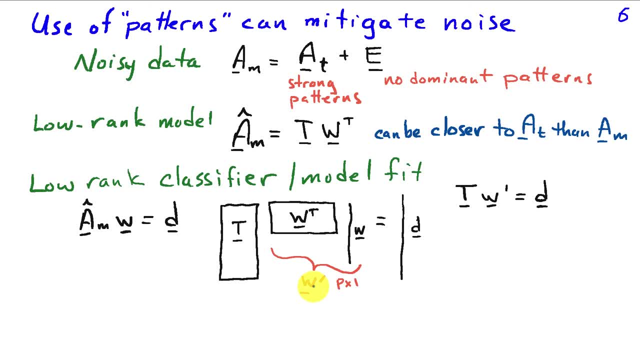 axiomatic. So we'll see a p-dimensional vector. We'll call that w prime. So I can restructure this problem to solve for w prime and my least squares problem becomes t times w prime being equal to d, And we can solve. 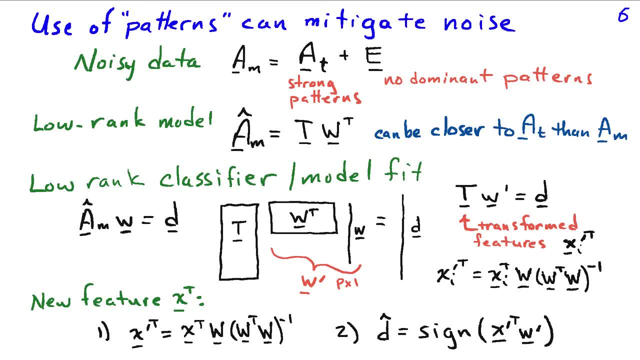 that problem using straightforward methods of least squares. In fact, if the columns of t are orthonormal, as sometimes is the case, then this is a particularly simple least squares problem to solve. Now, these rows, the matrix T, I can think about those as transformed lower-dimensional features. So if I had the 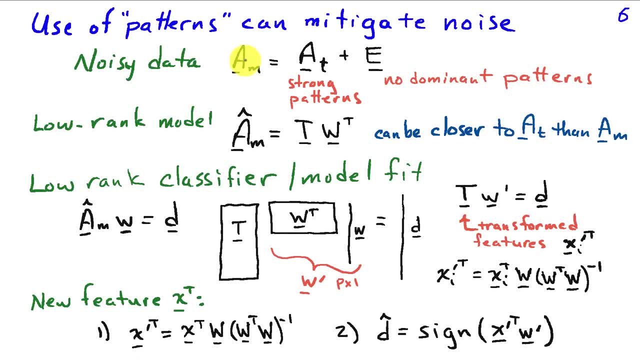 original rows in a sub m, let's say the rows of that matrix were features x i transpose. then these transformed features, we'll call those x i- prime transpose, and you can show that the relationship between the transformed features x i- prime- transpose and the original feature x i- prime transpose.